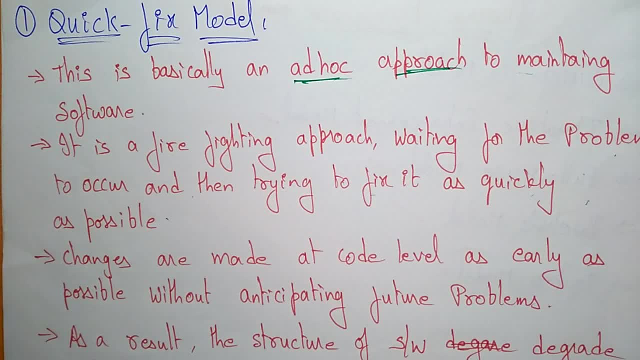 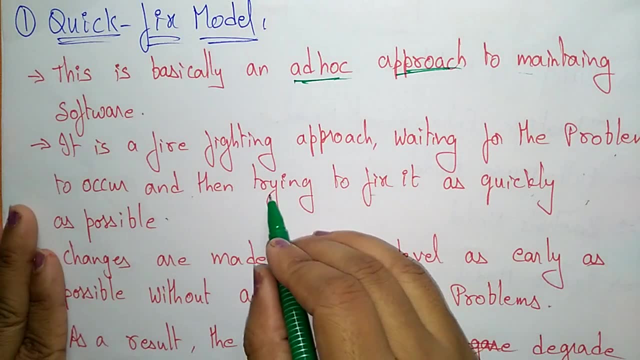 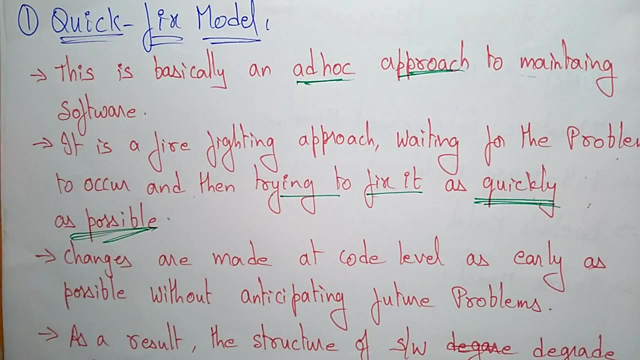 quickly as possible. so here the quick fix model is always waiting for the problem. is there any problem is occurring or not? suppose if there is problem is fired, then it trying to fix it, trying to fix it as quickly as possible. so that's why we call it as a quick fix model. 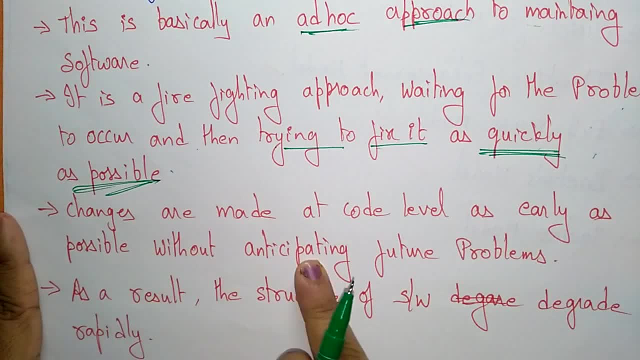 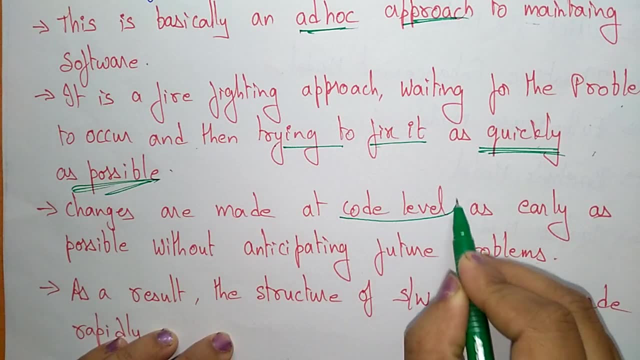 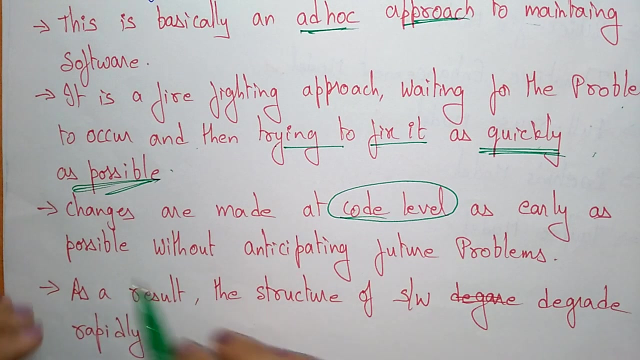 so changes are made at code level as early as possible without anticipating future problems. so try to find out the problem at code level itself. okay, so before going to the testing, only try to find out the problem. whatever the changes are made at code level as early as possible. 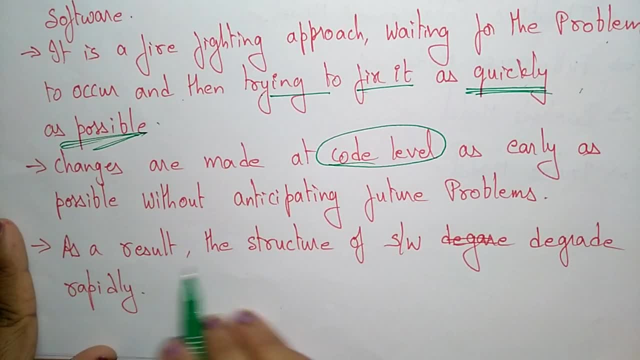 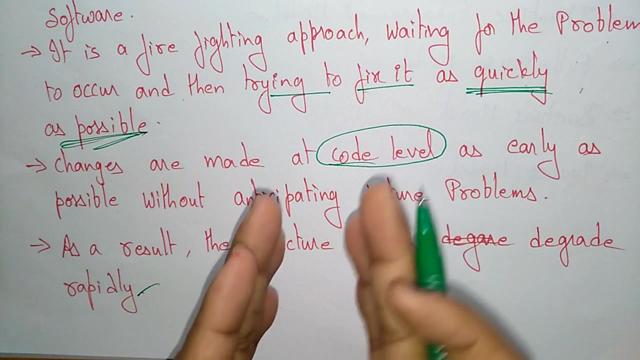 without anticipating future problems. so, as a result, the structure of software degrade rapidly because here every time we are just checking at the code level and we are trying to solve then. so it always the result of the structure of software degrades rapidly because it is not going forward. okay, whenever you're following the quick fix problem, it is our structure is not. 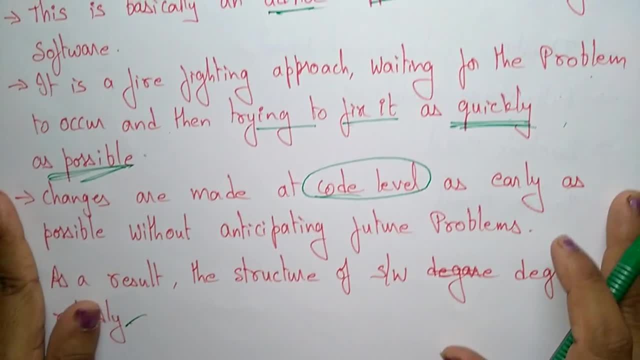 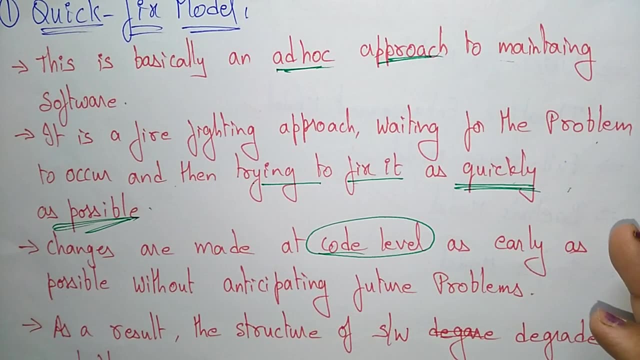 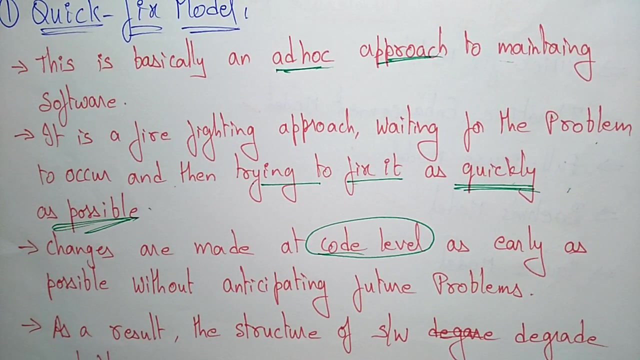 moving forward. so if it is the small projects, it is okay. so when you are dealing with the large projects, it is difficult to follow this type of model. means it difficult to maintain this type of model? okay one only for the small or small projects or small organization you can go for. 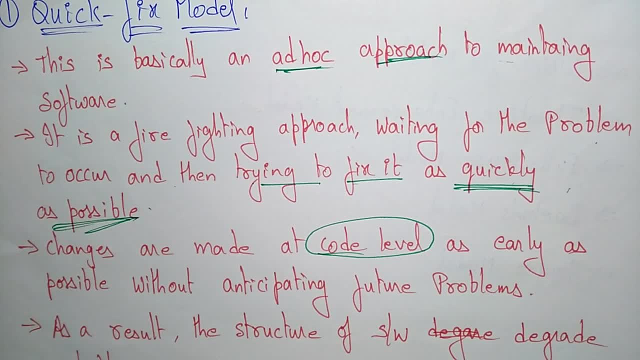 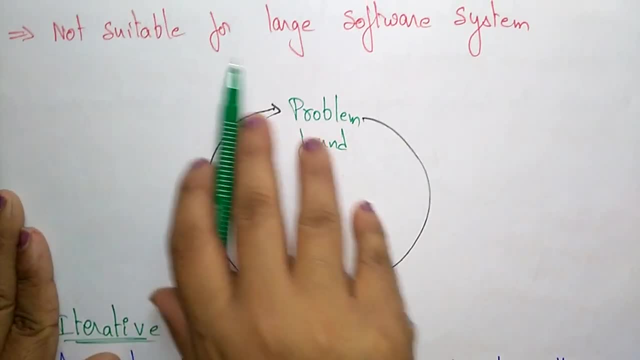 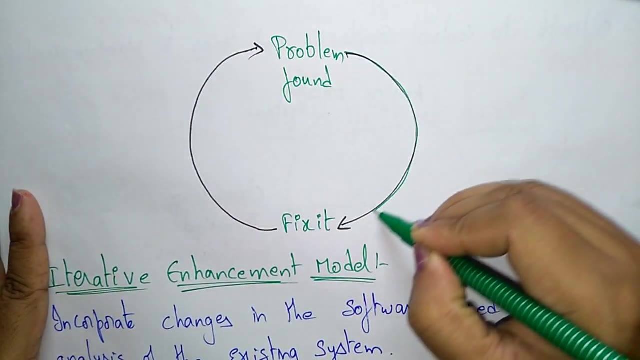 this quick fix model. okay, now let us see. this is a quick fix model. and one more thing: this is not suitable for large software systems. so whatever now. i said now. so whenever the problem is found, try to fix it before, before proceeding, that means after proceeding to the next step. try to fix the 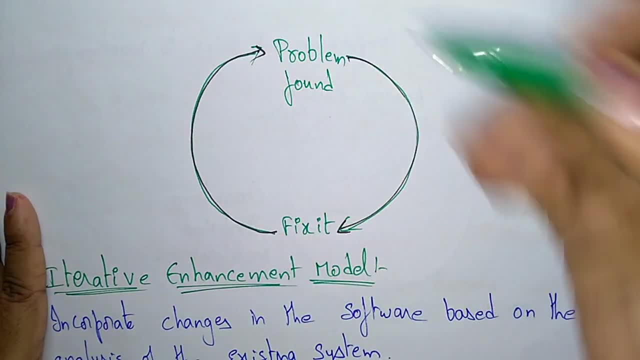 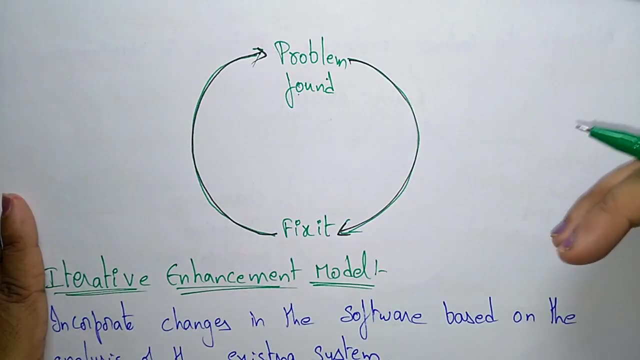 problem again, continue with the work. suppose, if again the problem is found, try to fix it. so, So here it is. continue, the loop is continuing. it is not going forward, okay. Otherwise, if the problem is not found, okay, it goes to the next step. 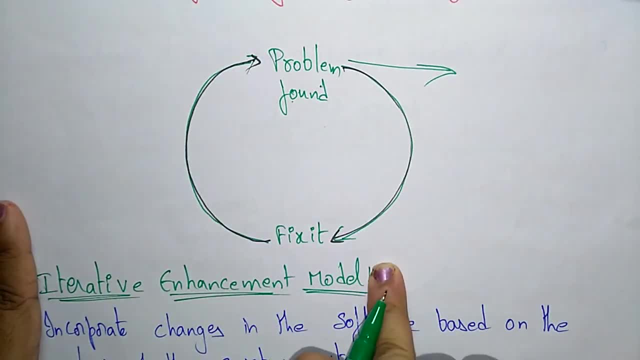 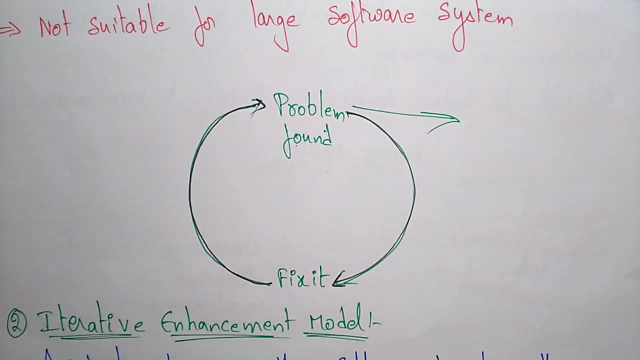 Until the problem was not found. the loop is rotating like this only So. that's why it is not suitable for the large software systems. If it is a small software means we can easily identify the problems and the problems will also occur at rare conditions. only for the small software systems, okay.